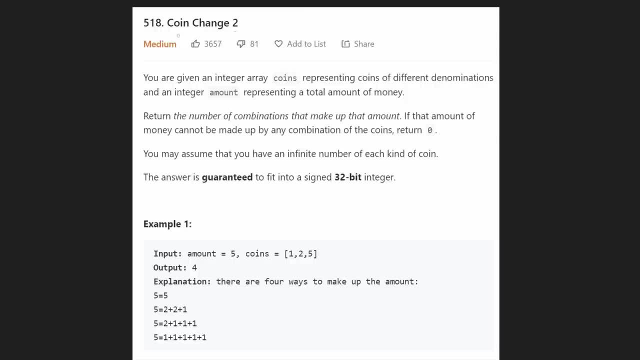 everyone. welcome back and let's write some more neat code today. so today let's solve the problem. coin change two. we already solved the first one and i'll link that somewhere on the top right of the screen or somewhere in the description. if you want to watch that video, you don't have to solve. 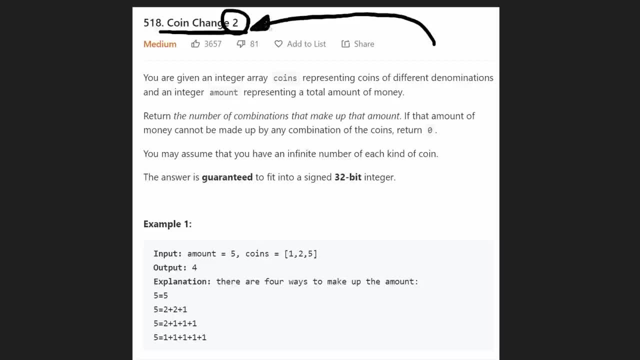 it before solving this problem, but it'll probably be easier to solve this problem if you do so. similarly, we're given a list of coins, each representing a different amount right, a different denomination, and we're given a second parameter, an integer amount, and this is the amount that. 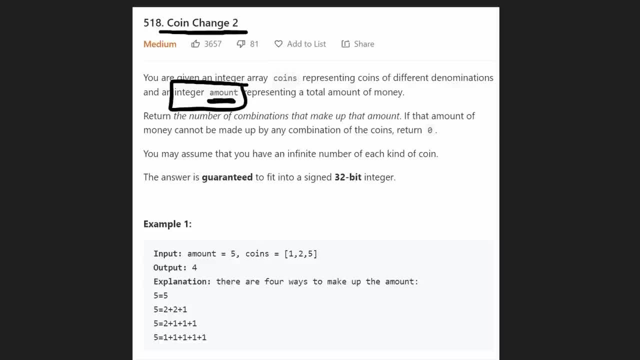 we want to sum up to. it's a total amount of money that we want to sum up to, given these coins. and specifically, we want to know, with these coins and this particular amount, how many different combinations are there that we can sum up to this amount? of course, if we can't ever sum, 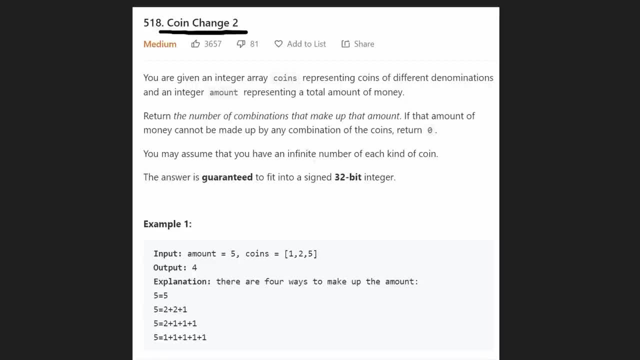 up to that amount, we can just return zero and we can assume that we have an infinite number of each type of coin. so i'm just going to select a put name and we want to multiply it by the number above the value of each coin. so i simply multiply, just that. we just calculate the overs on this and 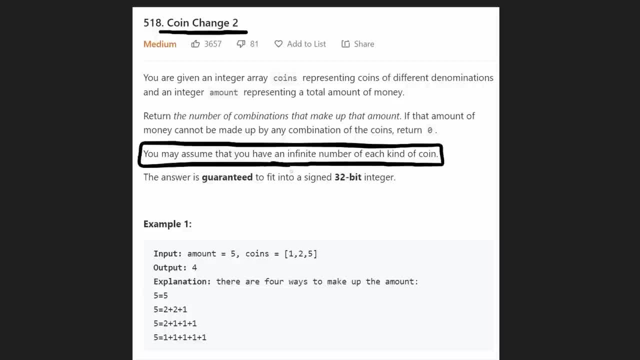 so that kind of hints to you that this is an unbounded knapsack problem, which i talk about that category of problem in one of my videos. i think it's called top five dynamic programming patterns, if you want to watch that video. and so this is kind of one example that they give us. 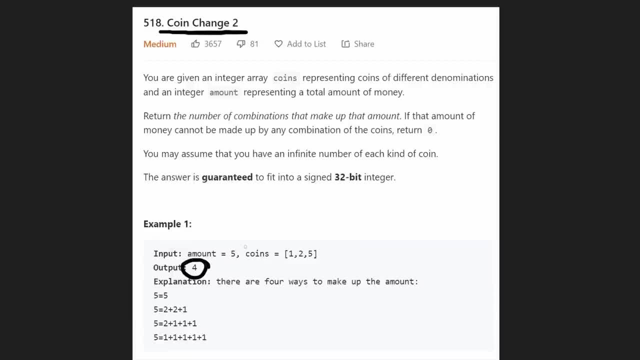 and you can go ahead and read it if you want. there's four different ways to sum up to the amount five: if we're given three coins- one, two and five- now when we say number of combinations, we can't reuse the same combination right. so if we get two, two, one, two, two, one, these three coins. 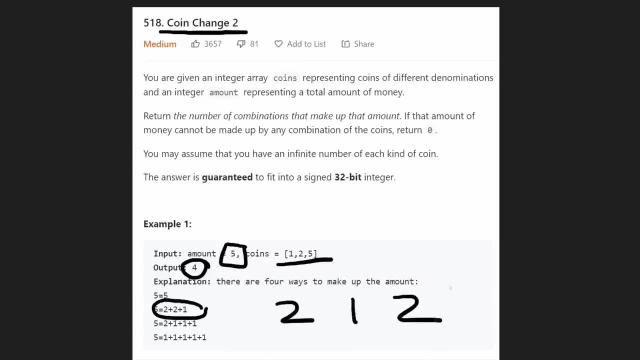 sum up to five. we can't just change the order and then call that a different combination. the order doesn't really matter. so now let's kind of get into the explanation. let's talk about the brute force explanation, which is going to be exponential with c to the power of n, whereas c is, let's say, 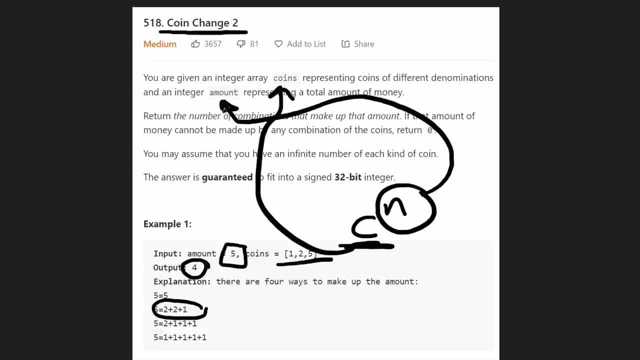 the number of coins that we have and n is the total amount that we want to sum up to. that's the exponential solution. we can use memoization on that decision tree to actually get the time complexity to be big. o of c times n. i'm actually just going to replace the variable c with m, so let's call it m to the power. 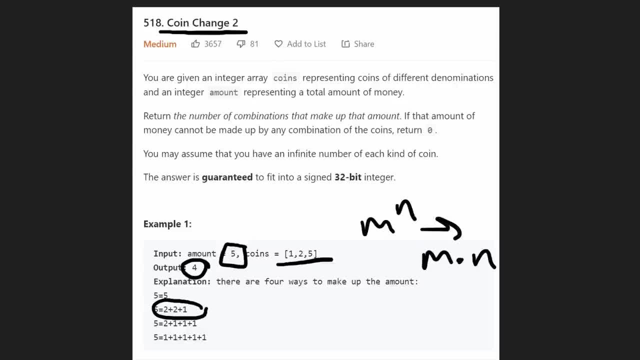 of n that can be reduced to m times n, this time complexity. that's the best time complexity we can do. but there is one optimization with memory complexity that's pretty difficult to come up with. but i'll kind of explain it to you. so let's get into that. so same example we're trying to get. 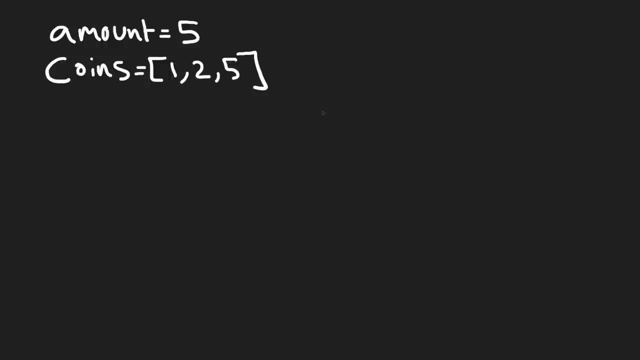 the amount five with these three coins. let's just think about the amount of coins that we have. so let's think about the brute force. so initially we have a sum of zero, right, we'll put that in a node. and we have decisions we can make. right, we're just gonna make three decisions? right, we can. 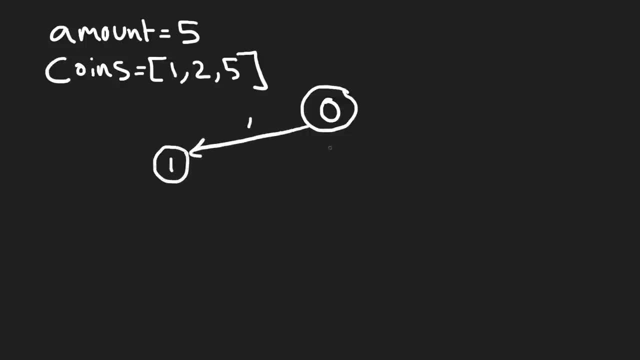 either choose a coin of one that that would give our sum to be one. we can either choose a coin of two that would give our sum to be two. we could choose another coin to be five that would put our sum to be five right, and then we can continue this approach. the only thing is: how do we guarantee? 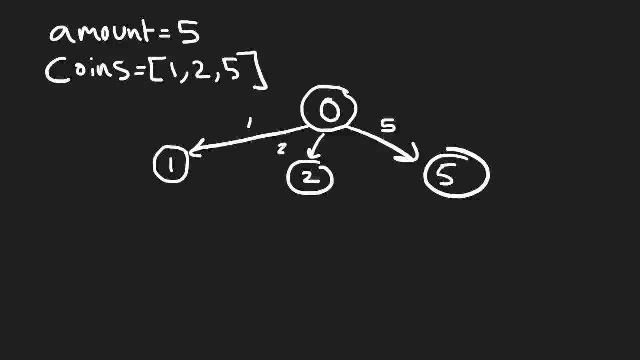 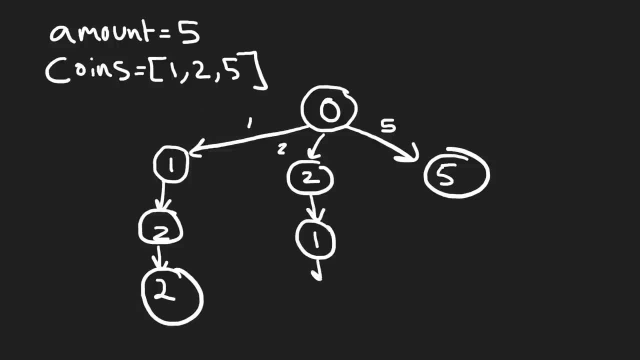 wanted. here we could do the same thing, couldn't we? we could get a one and then we could get a two. this is the same, uh, combination of coins, just a different order. right, we don't want to get into this case. so how can we guarantee with this decision tree that we won't ever get something? 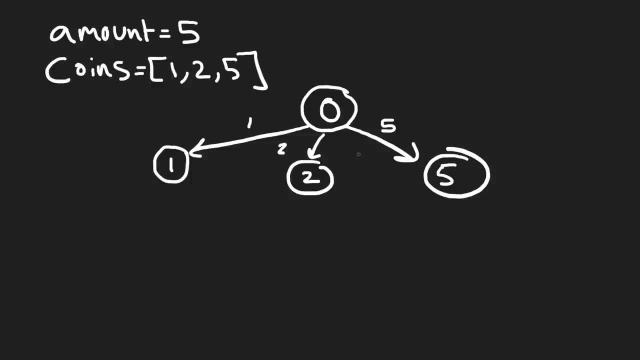 like that. well, how about, every time we make a decision- right, we made three decisions in the this case- we put some rules on that decision. how about, when we go down this path, we are allowed to choose. we chose a one right. we chose the coin one, and we're allowed to choose any coin that we. 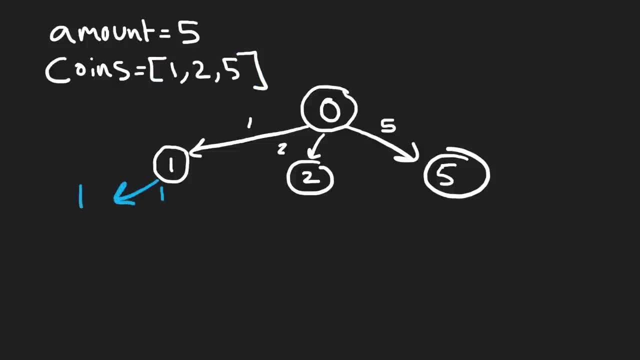 want. right down this path, we can continue to choose a one, we can choose a two, we can choose a five if we want, but we want to make sure that this never gets any duplicates as this one. so how can we guarantee that? how about this path can never choose a one? how about we just don't let us? 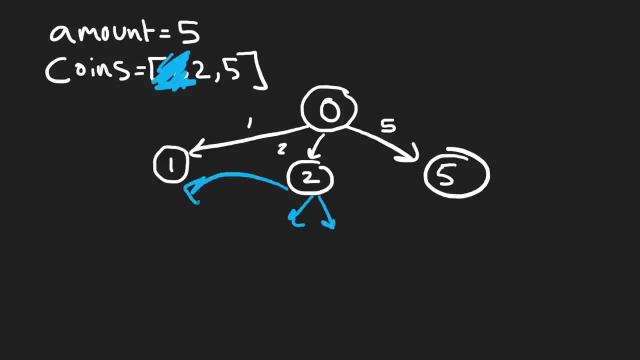 choose ones anymore down this path to make sure that we never have duplicates on the other side of the decision tree. right, we're free to choose any twos and any fives that we want, but we just can't choose ones. hopefully it makes sense why that guarantees that we won't have duplicates. 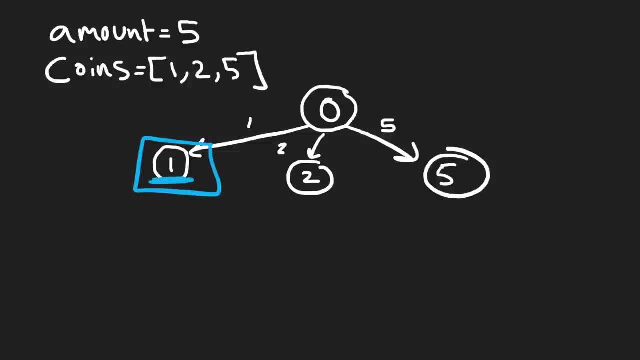 right, because this path has at least one one right and this path will never have anyone. so obviously neither both of these paths will never have the same combination. i hope that makes sense. and similarly, over here, when we choose a five, we're gonna, we're gonna say: 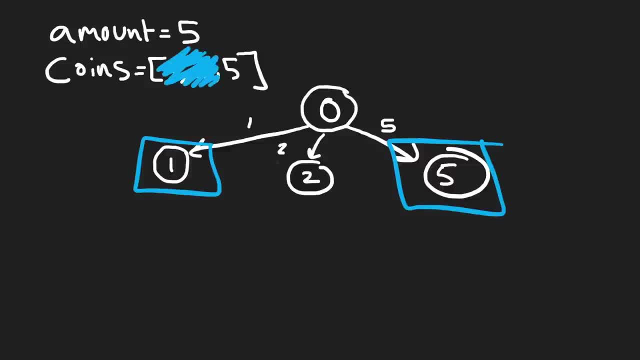 okay. we're not allowed to choose anything except fives right. we can't choose ones or twos. that'll guarantee that these two are not the same right, because we have a two here and we'll never have any twos down this path, so they'll never be the same. so that's the main idea of how i'm going to. 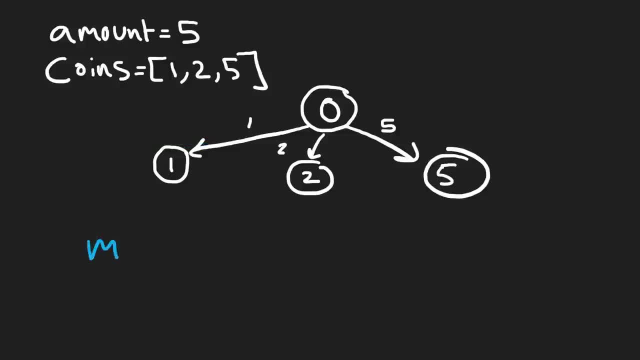 eliminate duplicates. so now we've gotten to the point where we have the m to the power of n solution, right? the base case is going to be: if we get to the amount, so you can see, on this path we already reached the amount right, we have a total of five. that's exactly the target that we're trying. 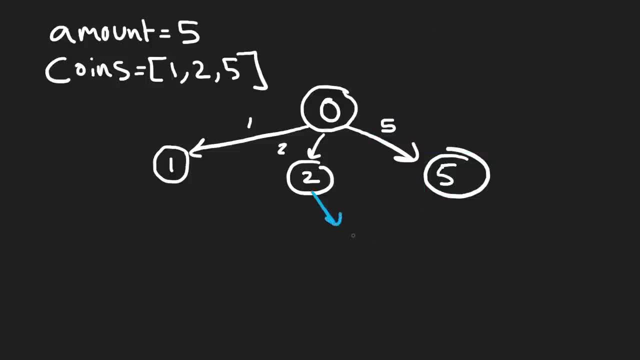 to get to now. let's say we're going to choose a one, right, so we're going to choose a one, and we're going to choose a five over here, right, we chose a coin of five that would put our total at seven. if we go over the total amount, then we're going to stop, right, then we're just going to return zero. 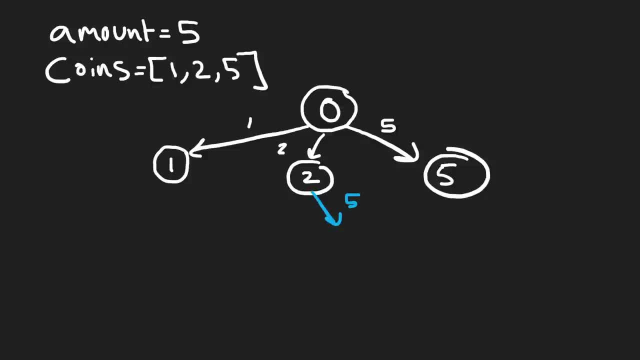 and then stop going down that decision. so those are the main base cases. and, by the way, how are we going to implement that idea of if we chose a one or chose a two, we're not allowed to choose any other certain coins? right, we're going to be maintaining a pointer. uh, let's call it i it's. 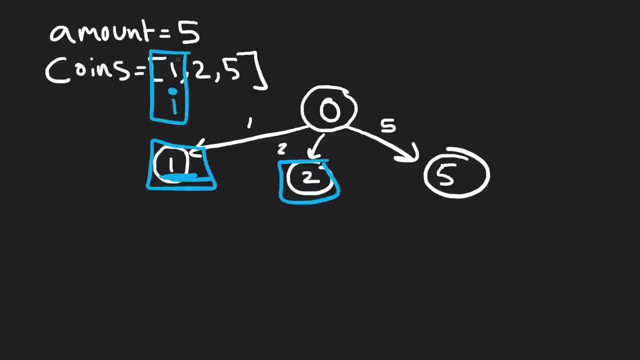 going to point at some index of coins, right? so if we chose a coin of one, then our index is going to be here, right at the coin of one, and then we're going to choose a one, and then we're going to choose a coin one, and if we chose a coin of two, then our index i is going to be at this coin two. 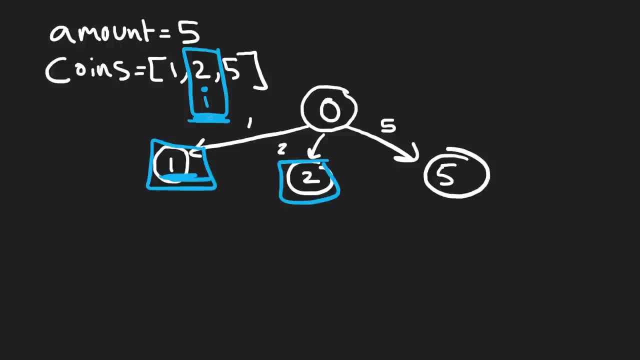 and what? when our index is at a coin, then it basically means that we're not allowed to choose any coins with an index less than it. so basically, anything on the left side of this coins array, on the left side of our pointer i. we're not allowed to choose those coins, right? so that's. 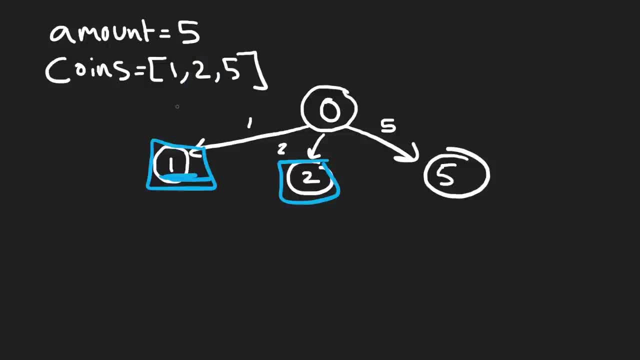 how i'm going to implement it in the code. and this is important because now that we actually move into the memoization solution, the memoization solution where we're going to be caching the repeated work, because when you look at this decision tree, it's going to be pretty inefficient, right, like i said, it's going to be m to the power of n. 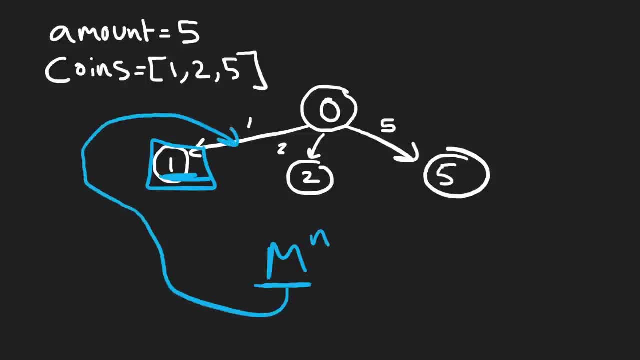 where m is the number of decisions we can make, in other words, it's the number of coins that we have, n is the total amount right, because the amount is what's going to determine the height of the tree. so when we implement this recursively- let's call it dfs- we're going to pass in two parameters: one: 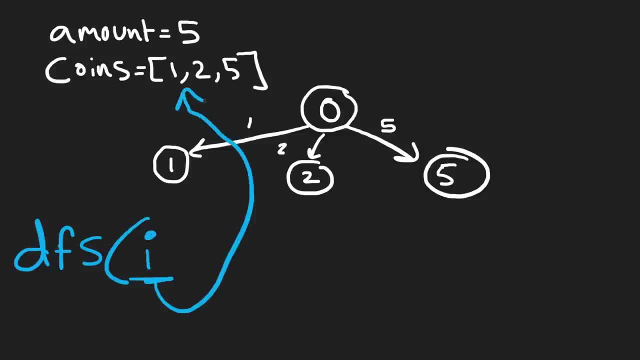 parameter is going to be i, which is going to tell us what index we're at in coins. it could be, you know, any of these positions and we're going to pass in a second parameter, let's call it a, which is, whatever the current amount happens to be- remember, if the amount ever goes over five- which 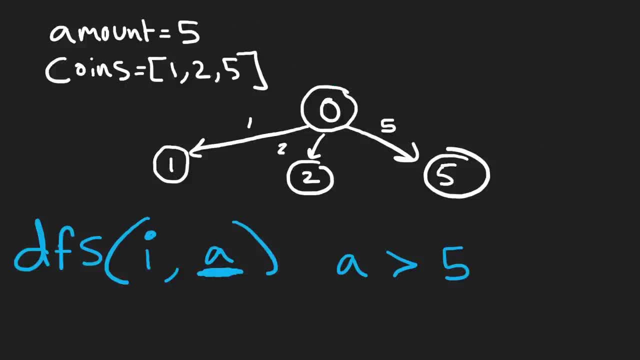 is you know the target that we're trying to do, then we're going to stop right. so, basically, the total number of about possible values a could be is going to be whatever that target value is. so when you look at this right, how many different combinations could this dfs be called? basically, 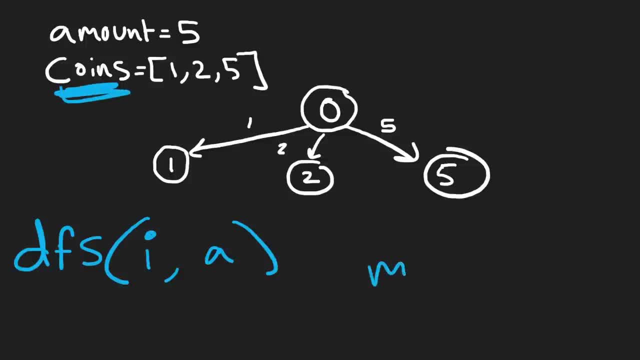 the total number of coins that we have, right, let's call that m, and the total amount that we're trying to sum up to, let's call that n. so the total possible number of ways this dfs could be called is m times n. so if we cache the repeated work, right, if we 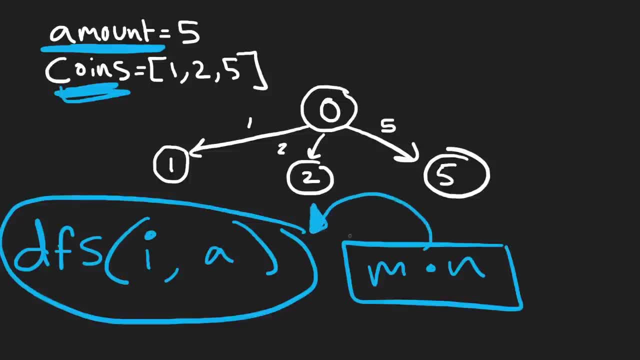 call it with the same values. we don't want to have to recalculate the same thing. if we call dfs, let's say, uh, on index one, and let's say our amount happens to be two and we call this multiple times. we don't want to have to recalculate all that work. so we can do caching with that, so that's. 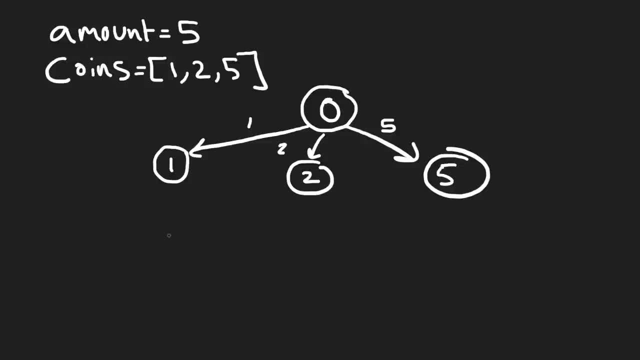 pretty much where i'm. we're going to be able to do all of this to make the shambles and the schema really smart, but then we have to do this and it's not going to work because we don't want that to be a thing to do. so at this point we've gotten to a solution that will pass on leet code the time. complexity will be m times n and the memory complexity will be the same. but now i'm going to show you the dynamic programming solution, which will actually have the exact same time and space complexity, and then i'm going to show you a slightly more advanced dynamic programming solution. which will actually reduce the memory to, instead of being, o of m times, and it'll actually be o of n. this is one of the reasons why dynamic programming solutions provides a completely勝利. if you have a problem with a space on combination, so that's right. and then next step, number of times. we're going to figure out the correct number of times and we're going to 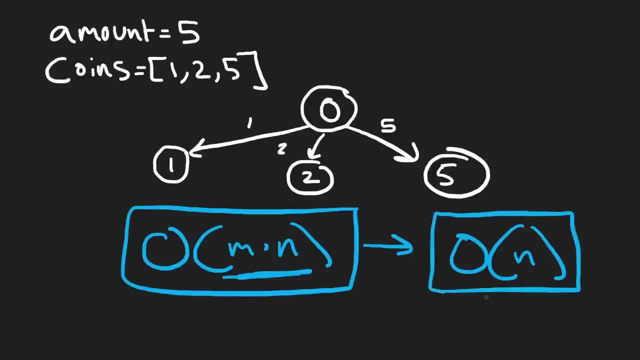 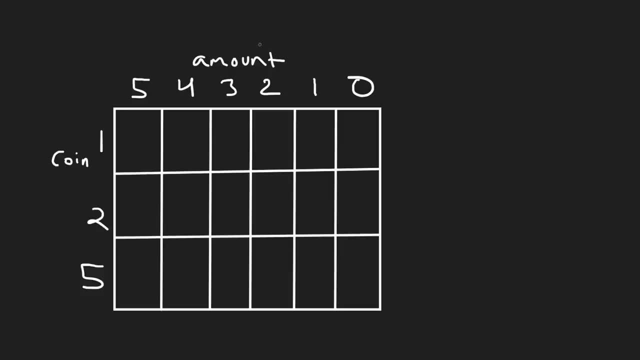 dynamic programming is important because sometimes the dynamic programming solution can actually be more efficient than the recursive memoization solution. So if you want to check that out, continue. So now let's do the dynamic programming solution. You can see, I drew a 2D grid where we 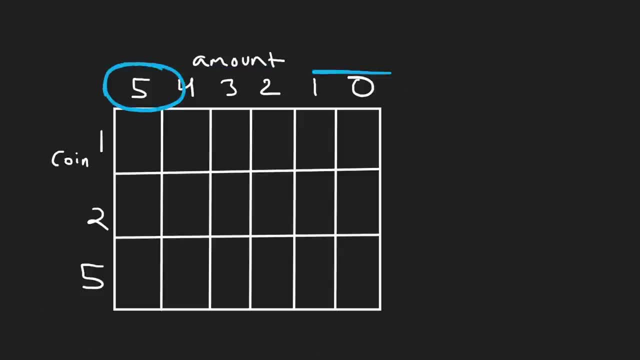 have one dimension being the amount, the, you know, zero from zero all the way up to five, and one dimension being the coin. We had three different coins, one, two, three, And we know the base case is: if the amount is zero, right, And what value are we going to put in here when? 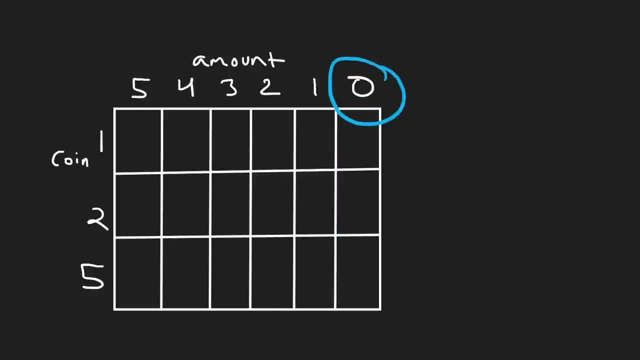 the amount is zero. How many different combinations is it that we can sum up to zero? Well, the base case is: let's just put it as one right, Because that's what's going to make the math work out And it kind of makes sense, right? How many ways can you sum up to zero? Just one right, Regardless. 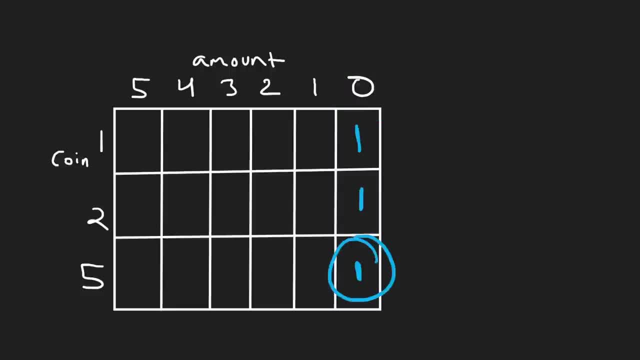 of which coin we start at. So what does this position mean? It means that if we could only choose from this single coin five, how many different ways could we sum up to zero? It's going to be one different way, right? And this position is going to mean if we had two coins, 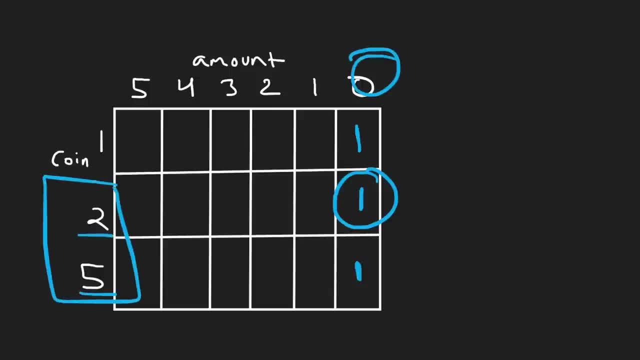 available to us? two and five. how many ways Could we sum up to the amount zero? It's going to be one right, And so on and so on. For an arbitrary position like this, the question is: how many different ways can we sum up to the amount? 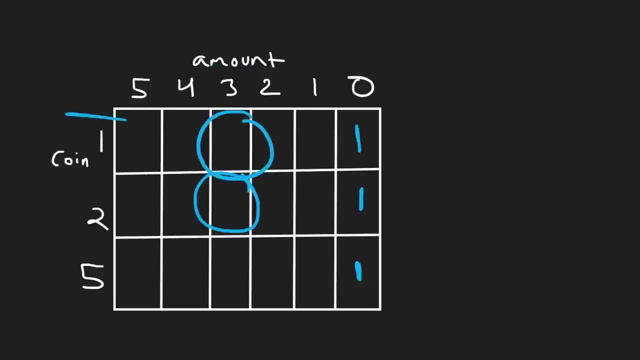 three using these two coins. From here, it would be using these three coins, right? So what order would it make sense to compute these values? Probably bottom up, right. That's why they call this bottom up dynamic programming. We're going to start here and compute the value that goes. 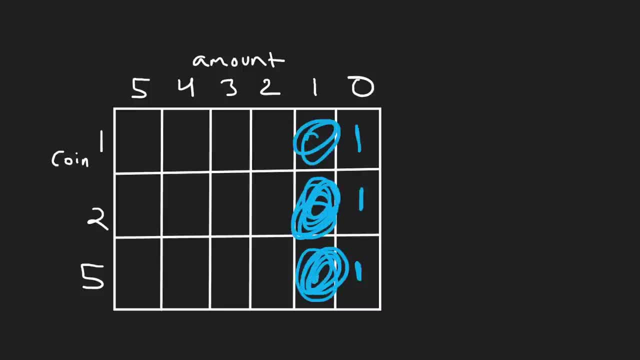 here, Then we're going to compute the value that goes here and then here, And then start from here and then do the same And, looking at it, since we're doing it in this order, you're probably thinking I probably should have rotated this. Instead I should have put the. 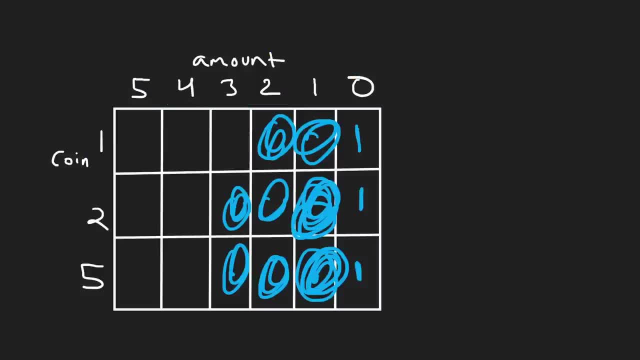 amount over here and the coins over here, because then we can actually compute it like this. And you're right, but there's actually a way that we can compute it like this that I'm going to show you. And actually this way, if we do it in this order, is going to be better memory complexity. 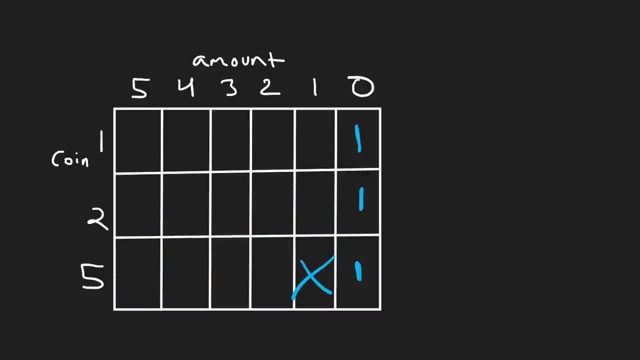 Let me show you why that's the case, though. So let's say, starting from this position, right, We're trying to sum up to the amount one, If we use a coin, we can only choose one coin that's available to us. right, We can choose a five coin. What happens if we use a five coin? Then our 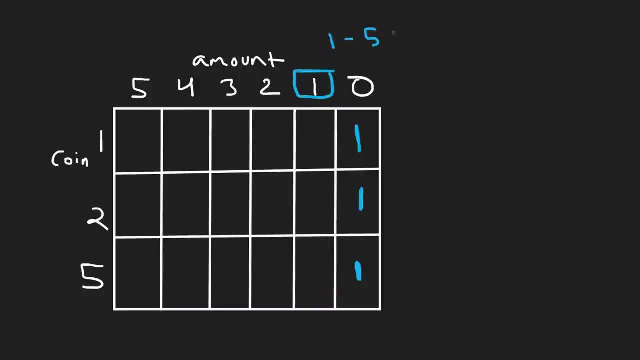 amount that we're trying to sum up to is going to be one minus five. right, That's going to put us at negative four. So from here I'm going to go to negative four. Now, that's out of bounds, right. 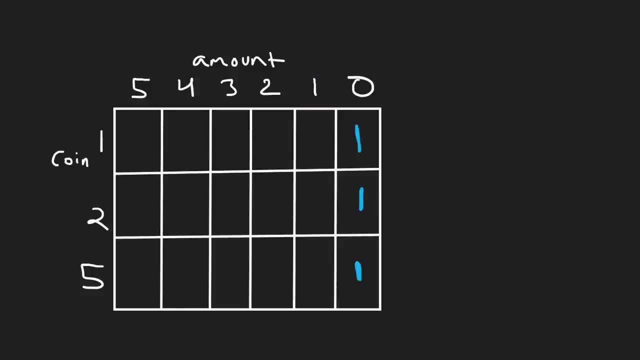 So that kind of tells us that there's zero ways to sum up to the amount one if we only have a single five coin available to us. Next let's compute the value that would go here. So we have two coins available to us So we can choose to use the two coin. What happens if we use the two? 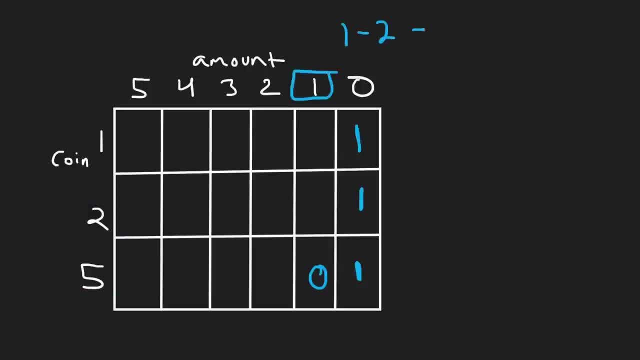 coin. Well then, our amount one is going to be one minus two, which is going to be negative one, right? So if we're trying to get the value here, then our arrow is going to go over here out of bounds, which is negative, right? So that doesn't work. And that's if we choose the two coin, If we 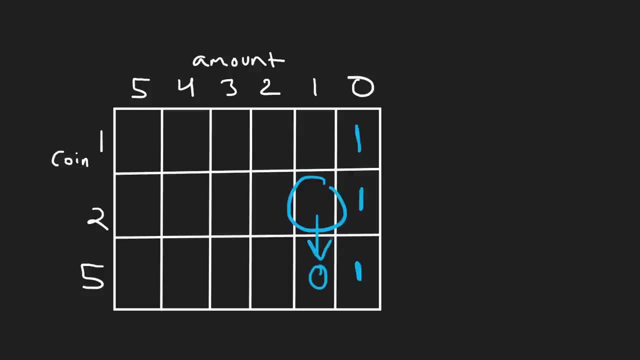 choose the five coin. what are we going to do? Well then, we're just going to look directly below us, because we're still solving the same problem. amount equals one, but in this case, we're choosing not to use the two coin. we're just going to use the five coin. 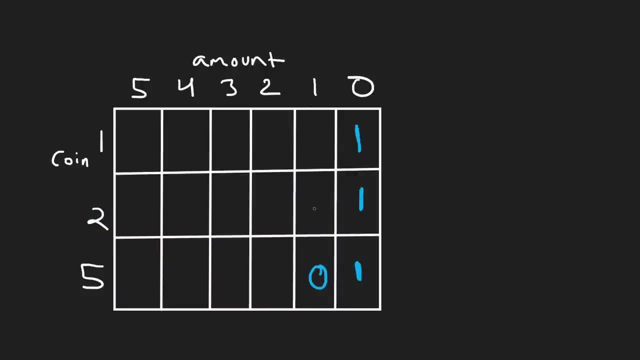 But we see that that's a zero value down here, So in the end we'll also end up putting a zero here, And from here we're going to do the same thing. In this case, we have three coins available to us. 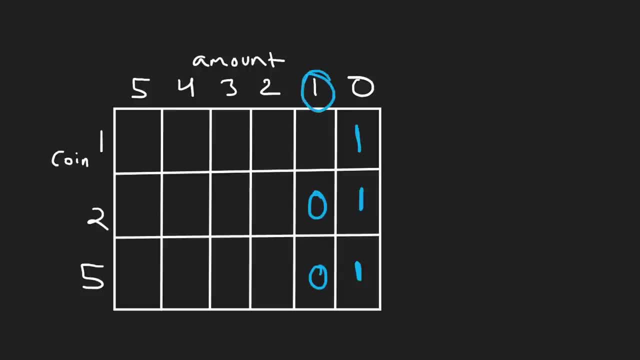 If we use a one coin, what is that going to put us? Well, we started at, we're trying to get to the amount one. If we use a one coin, we'll do: one minus one equals zero. So okay, then from here. 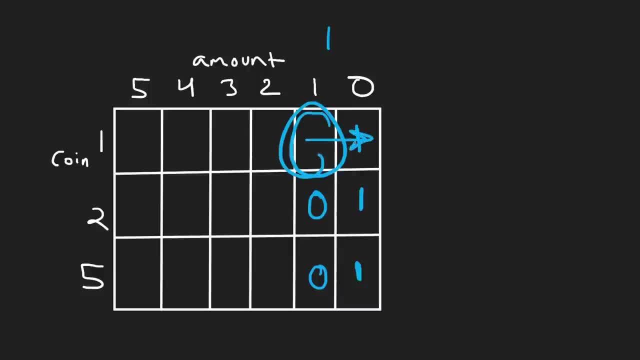 we're going to, you know, go to the, to the spot that has a value of zero. right, That's directly to the right of us, right, That's where zero is. So then, we're going to take this value. 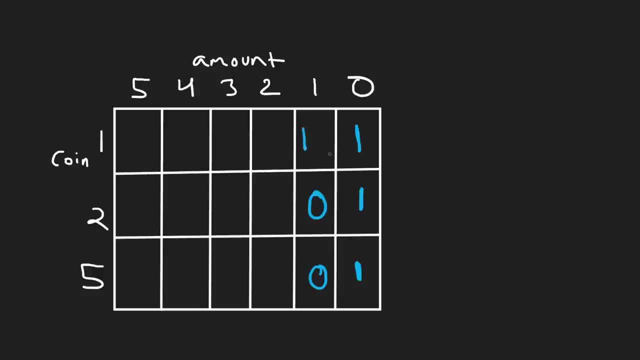 add it to this position, right? So one is going to be added here, But we don't have to choose this one coin, right? We could actually choose the two coin we can ask. okay, instead of choosing one, what happens if we try to sum up to the value one with two coins available to us In that case? 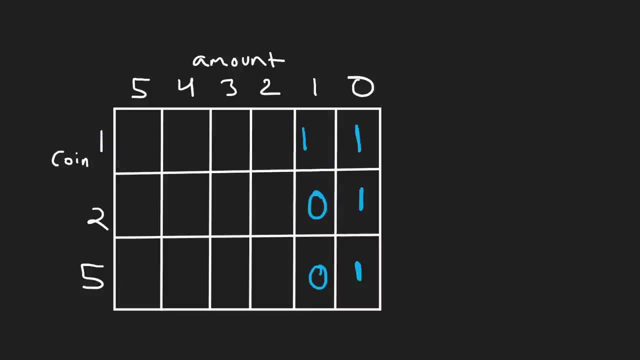 we look directly below us And we see that there's a zero there, And we add zero to this position, one plus zero will just be one, So we can leave a one in this spot. So, and then you can kind of just continue doing the dynamic programming just. 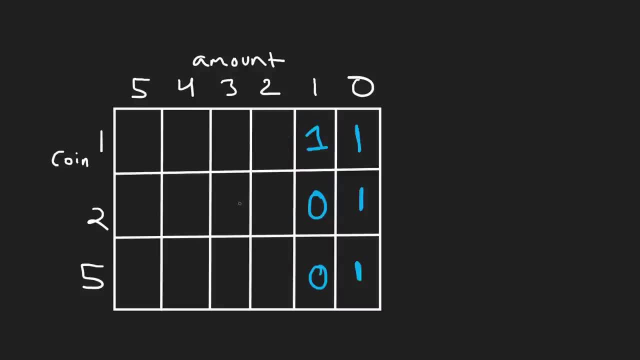 like this. One thing you might notice, though, let's assume for an arbitrary position like this one: if we use the two coin, that'll put us amount is four, we'll move two spots to the right where amount is two right, So we're looking all the way to the right. we could also say, okay, we're not. 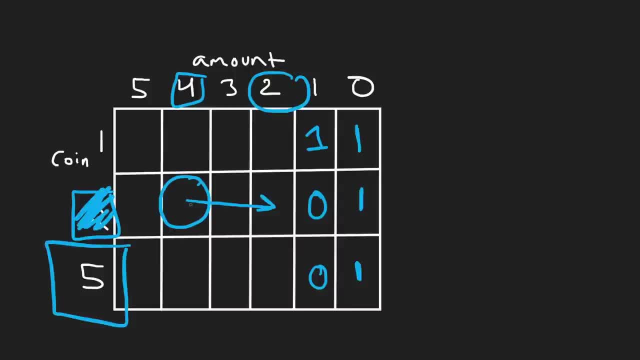 going to use the two coin, right? We're going to use all the other coins. In that case, we'd have to look directly below us, right? That's perfectly fine. This, this, perfectly works. But one thing you're noticing: for a arbitrary position like this one, we have to look both to the right. 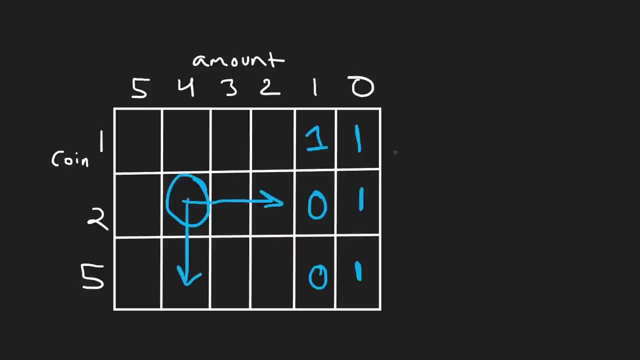 and we have to look below. What does that mean? That means, potentially, we have to have the entire two dimensional array in memory, Because when we're looking directly to the right of us, we're not just looking one spot. we could be looking two spots, three spots, five spots. 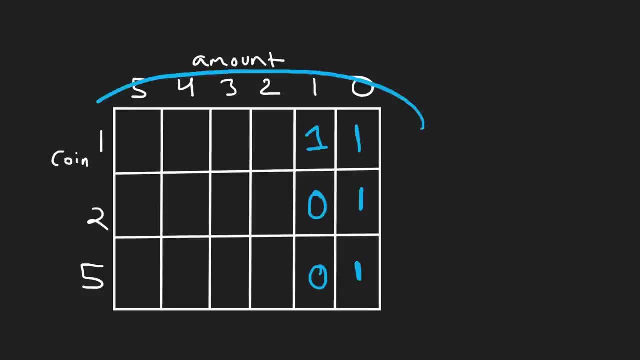 right, depending on what coin value we have. So in that case we're going to have to have this entire two dimensional grid in memory. there's actually a different way to do that, So we're we can do this problem if we compute this in this order right from here. in that way, we won't have 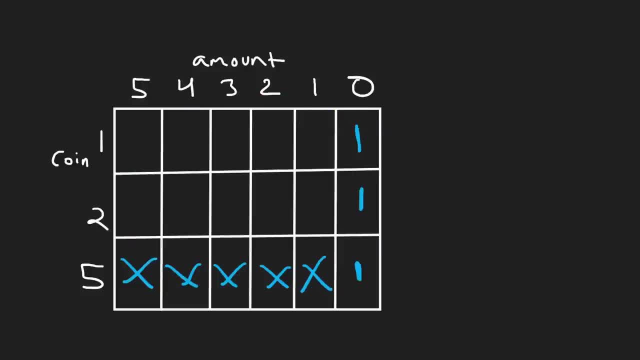 to have the entire grid in memory, we will only have to have up to two rows. two rows like these will only have to have up to two rows in memory And a row will only be as large as whatever the max amount happens to be, which means the overall memory complexity in that case will be big O of. 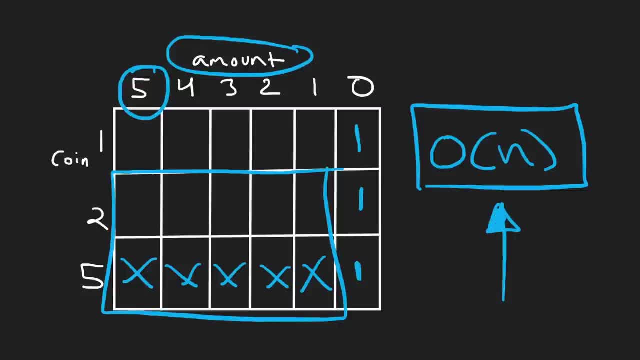 N. Now you probably don't need this solution to pass your interview, unless it's like a super hard interview and your interviewer is looking for it. But I'll show you both of the solutions. anyway. I'll show you the code for this. 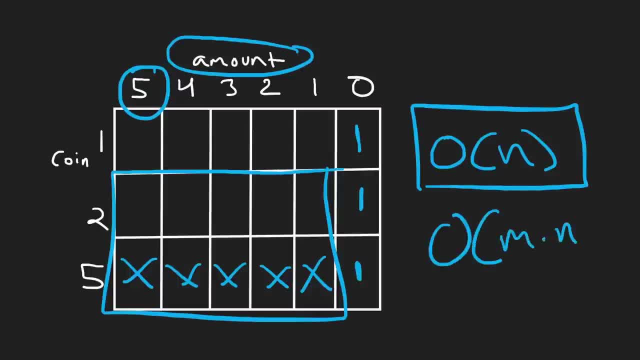 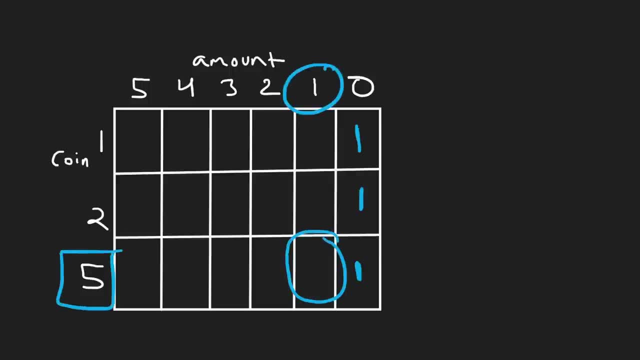 solution and the code for the memory solution of O of M by N. Okay, so in this spot we're asking the same question: if we only have one coin available to us, can we sum up to the amount one we can't write, because then we go out of bounds. So in this case let's just put a zero, Okay. 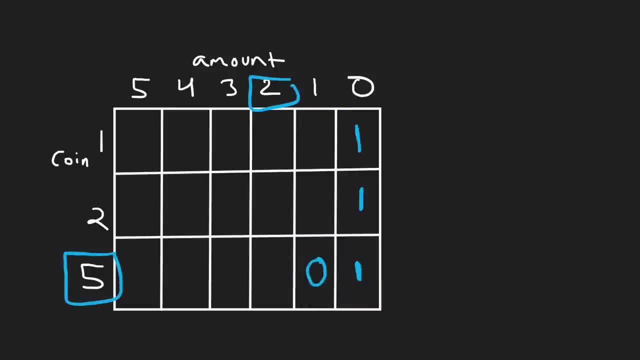 ask the next question: If we're summing up to amount two, with just one coin available to us, can we sum up to that amount? No, of course we can't, right? So, and that's going to be true for this position, right? Can't sum up to three. 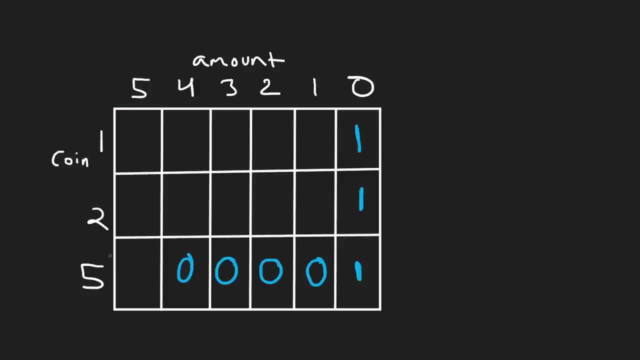 can't sum up to four either, But once we finally get to five with a single coin of five, what's going to happen? Okay, we use our coin of five, right? So that means we look five spots all the way to the right And over here in this spot we find a one is waiting for us, right, That's? 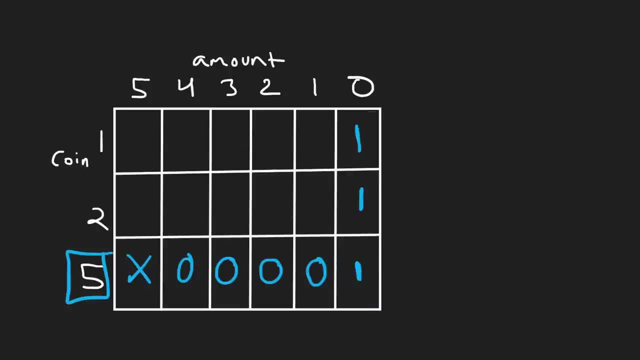 our base case, that's where amount is equal to zero. So we take that one and then we add it in this spot, right? So now we've done that. So there's one way to compute the amount of five if we only have a single coin available to us. But remember the actual problem. 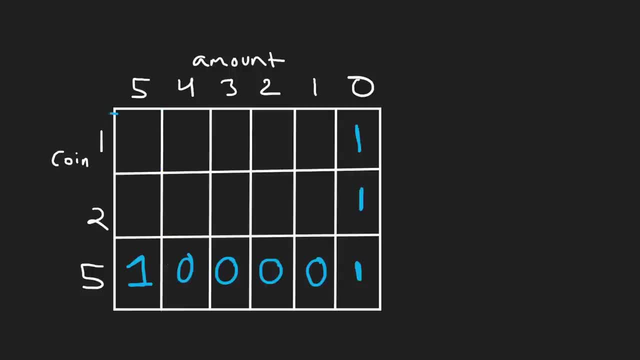 that we're trying to solve is all the way in the top left corner. if we had all three coins available to us- because we do- we have an unlimited supply of all three coins available to us. So how many combinations can we do to get to this amount? five? Well, let's continue row by row, just like I. 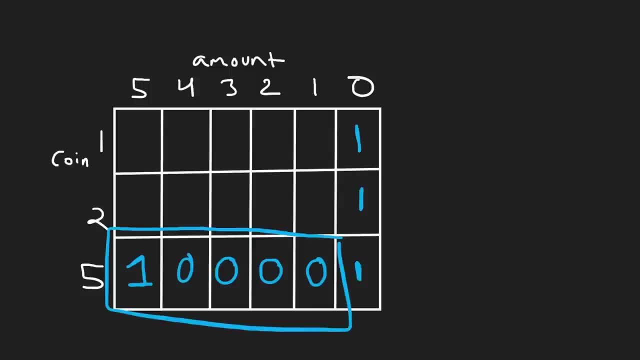 mentioned right. So now we will need to keep this row in memory for us to be able to compute this row. But once we're computing this row, we actually won't need this bottom row in memory anymore, And I'll show you why that's the case. So now if we had two coins? 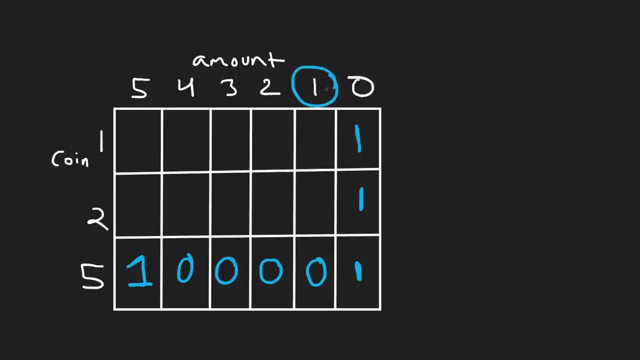 available to us. how many ways could we sum up to the amount one? Well, if we use a two coin, we'll go two spots to the right, which is out of bounds. So we don't put anything right so far, we're at zero. So if we 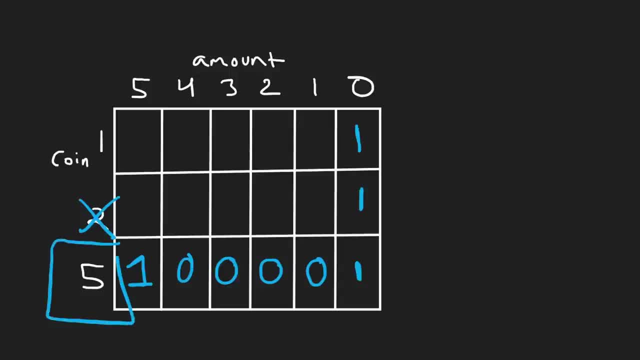 choose not to use the two coin, we say, okay, we're just gonna use all the remaining coins. then we look directly below us Again, we find a zero. So in this spot we say that there are zero ways to sum up to the amount. one if we have these two coins available to us, which makes sense, right? 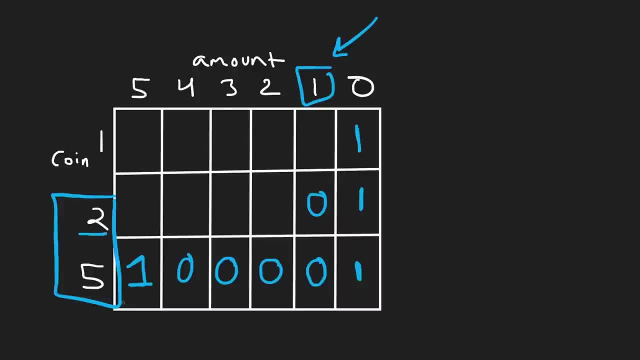 there's no way you can get a one if you have a two and a five available to you. Now let's do it in this spot. So if we use the two coin in this spot, we'll move two spots to the right, which will- we. 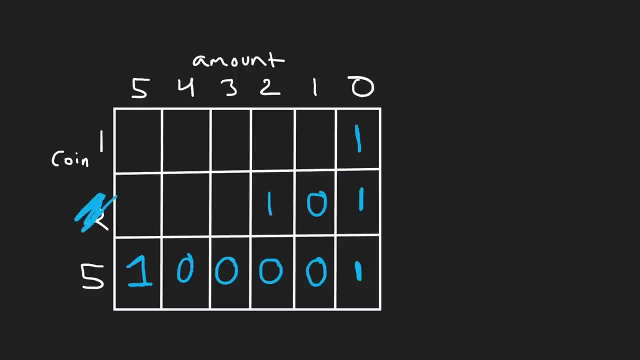 find a one here. right, So we can add a one here. If we choose not to use the two coin, we look directly below us, which is a zero, So we don't do anything in that case. Right, So we leave a. 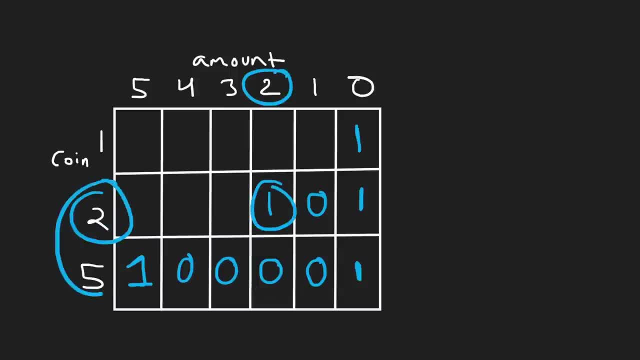 one here. There's one way to sum up to the amount two with these two coins available to us. And then I'm going to start going fast because I don't want to waste too much of your time. So in this spot we're going to look directly. 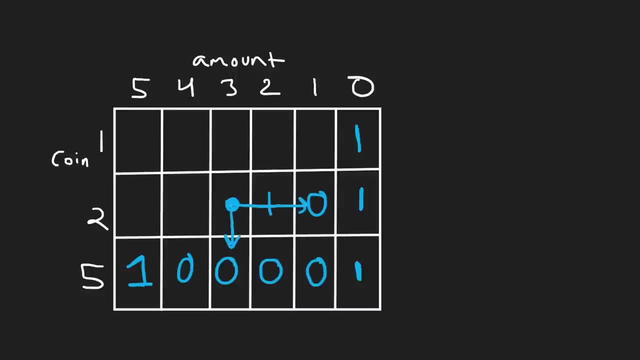 two spots to the right, which is a zero, or we're going to look directly down and that's a zero. So we'll still put zero here, Notice how we're looking multiple spots to the right, but that's okay because we have this row in memory. But when we look down, we're never going to look multiple. 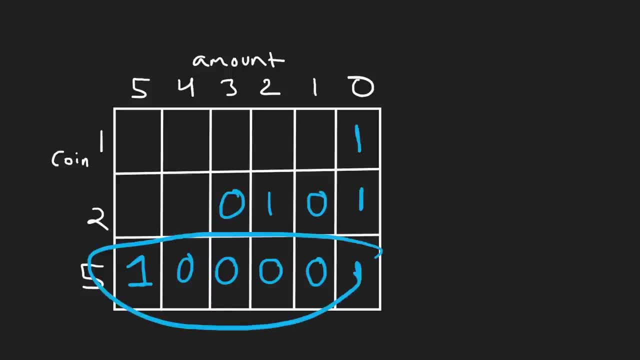 spots down. That's the key. That's why we only need O of N extra memory. So let's continue. So, from amount four, we're going to look two spots to the right. There's a one, or we'll look down. That's a zero. So we put one plus zero one here. Here again, two spots to the right. 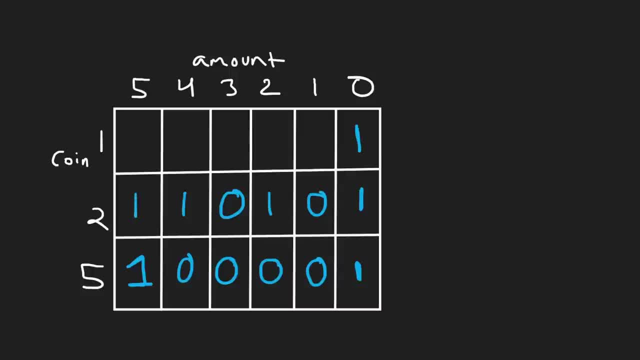 that's a zero, or one spot down, That's a one. So one plus zero, we get a one. Let's continue. So from here, we'll look one spot directly to the right, That's one. We'll look down, That's. 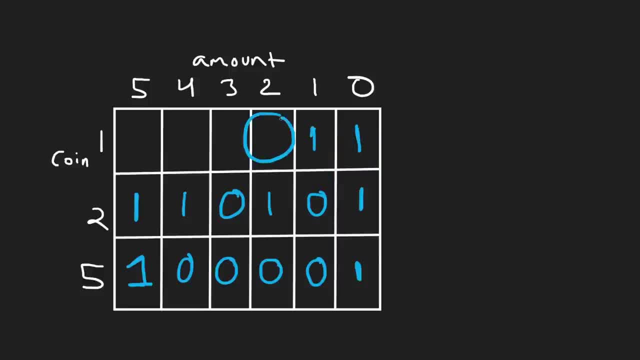 zero, So we'll put a one here Again. from here we'll look one spot to the right. That's a one. We'll look one spot down. Now we get a two right Because we're adding these two values together. that makes sense, right? because amount two. how many different ways could we sum? 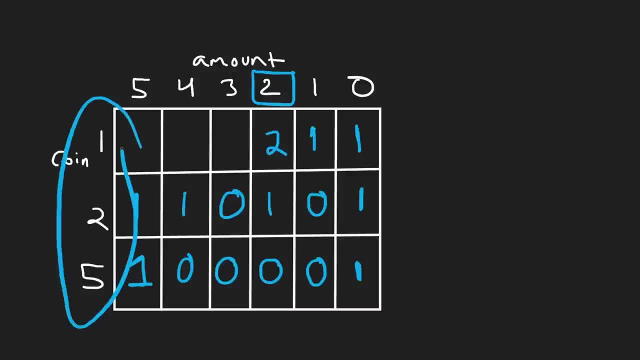 up to this amount. two, if we had all three coins available to us. there are two ways: right and from here, we'll look directly to the right, by one, two plus directly below, that's zero. so we'll put a two here, from here, again, directly to the right, directly below one plus two, that's going to be three. and 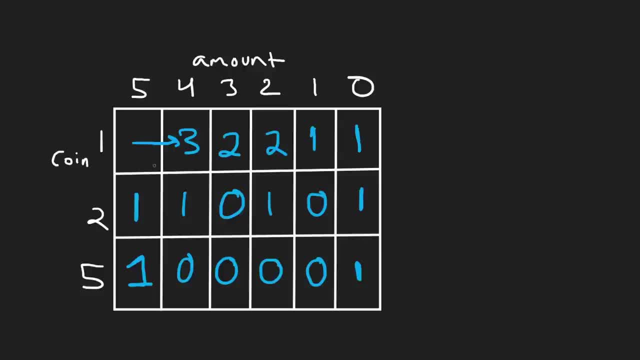 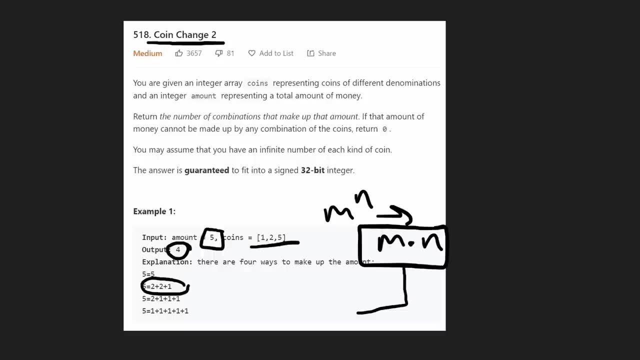 from here again directly to the right and directly below, that's going to be four, so we get a solution of four. is that correct? well, when you come back and look at the problem description with that example: yeah, that's what the amount was. that's good. now we're ready to dive into the code. okay. 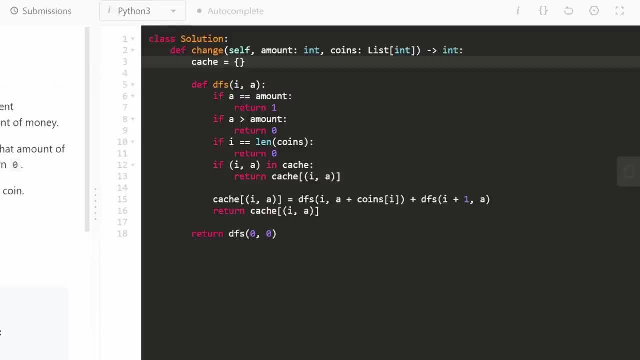 so now let's jump into the code, and since this video is probably already too long, i don't want to spend too much time coding it up, so let me just show you the code, and it will be in the description this time, if you want to copy and paste it or take a look at it. so this is the recursive solution. 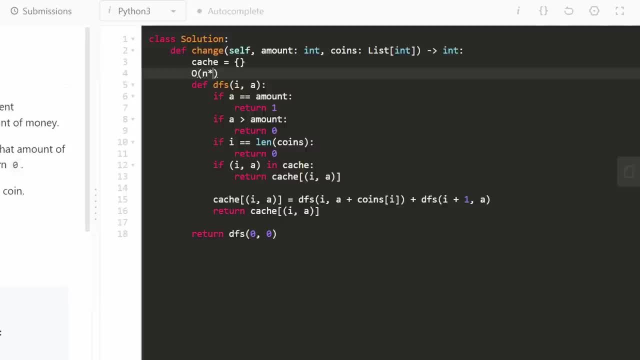 the time and space complexity is big. o of n times m. just like i mentioned in the explanation, you can see that we have a cap of n times m and we have a cap of n times m and we have a cap of n times m. in this case, the cache is the hash map. the base case is, just as i mentioned, right. so one is if we 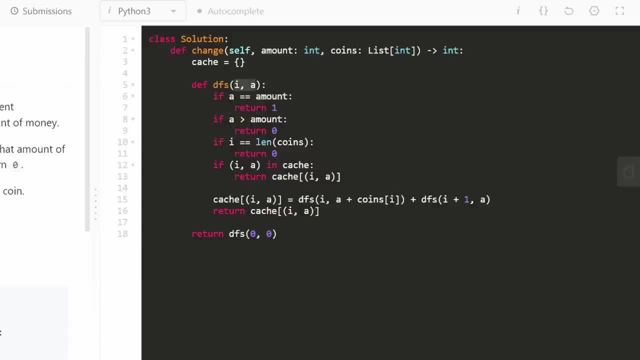 actually get to the target amount that we're looking for. remember, we're passing in two variables: the index and the amount a. if we get to the target amount, then we're going to return one if we go over the target amount. that's, that means we cannot possibly sum up to the amount we return. 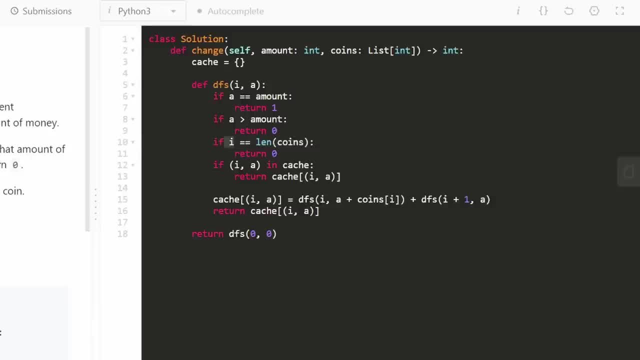 zero if we go out of bounds- meaning i is out of bounds, right. that basically means, now we, we decided that we don't have any coins available to us. uh, that's going to be. we're going to return zero as well in that case. and the fourth base case is if we've already computed this. if we've already computed it. 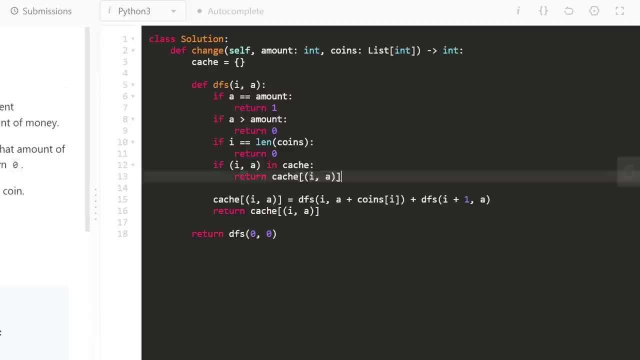 we can take it directly from our cache and then return it. the other case is now: this is the base case or not the base case? this is the recursive case. right, you can see i'm calling dfs twice. one is where i'm calling dfs is where we are choosing the coin that is at index i in that. 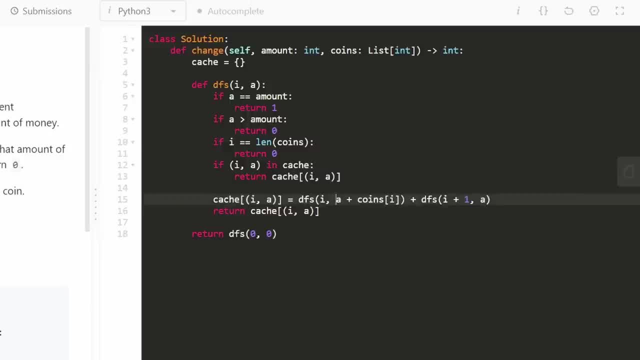 case we leave i just as it is and then we say: okay, the new amount that we have is a, whatever the amount that we previously had, plus whatever coin happens to be at index i. right, so we're choosing the coin at index i. that's one decision. the second decision is: if we skip the 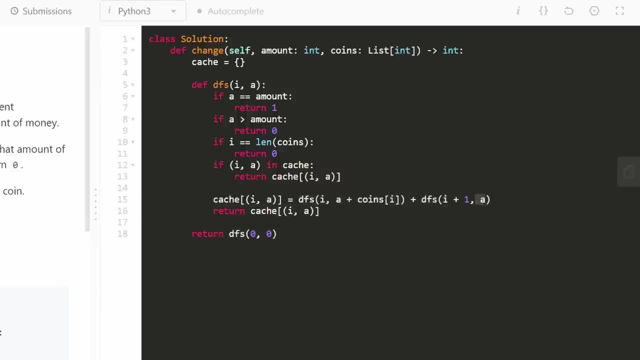 coin at index i. in that case, the amount stays the same. right, we skip the coin, so we don't change the amount, but we do have to increment our index i because we're skipping this coin right now. we're going to choose the next coin, so that's the main logic behind this, and then, whatever the result of, 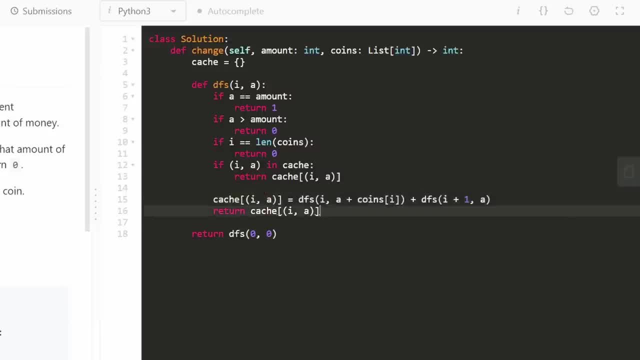 this happens to be. we're going to go ahead and throw it into our cache and then return the value from the cache, and so that's the entire dfs. all you have to do is call the dfs and just expos it to your caches. honestly, let's get started. 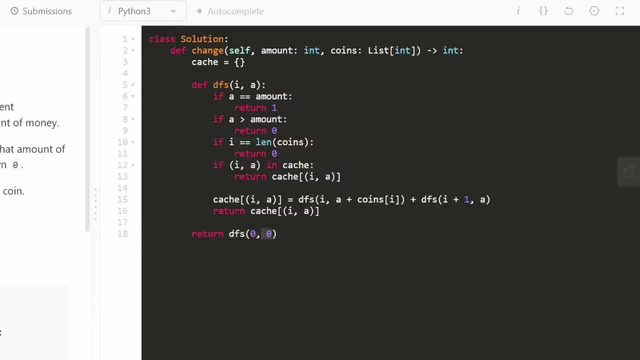 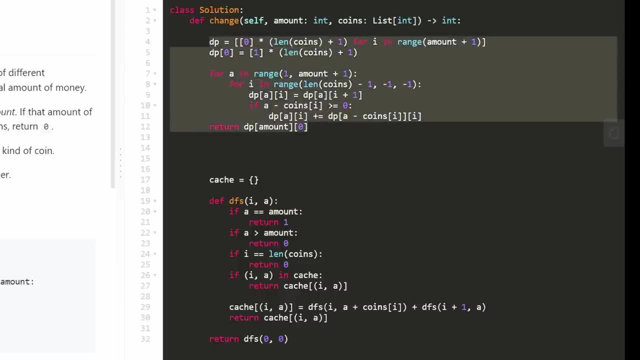 starting at index zero, starting with our amount being zero, and then we can just return that result. right up above now i've copy and pasted the dynamic programming solution where we had to use two dimensions of memory. so this is the same memory complexity: big o of n multiplied by m. 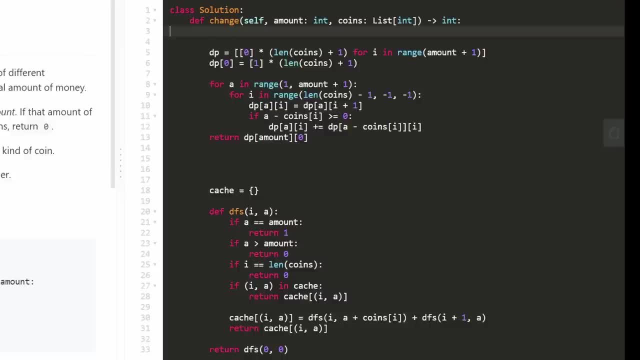 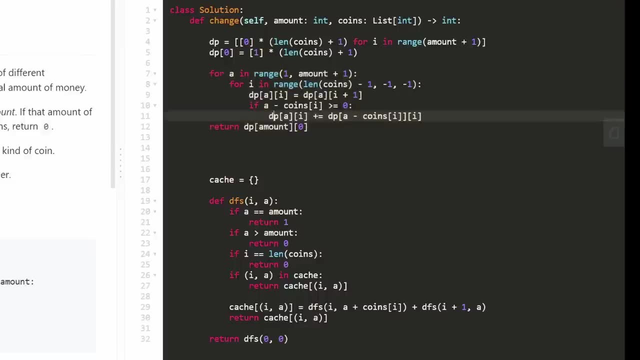 right, this is the one that was suboptimal for dynamic programming. so you can see i'm using two dimensions for the dp cache, and then the logic of this is pretty much the same. as i showed, right, we're going to be going from starting at amount equals one. uh, we're going to see how many different. 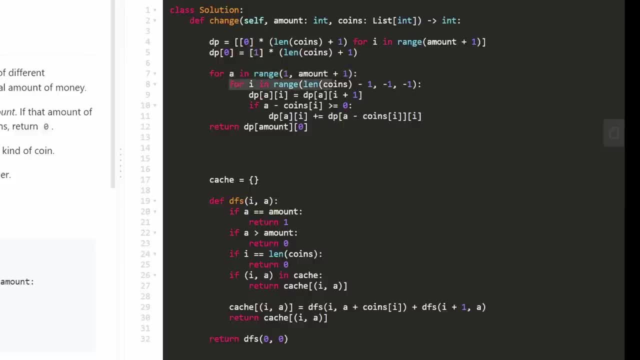 ways can we sum up to that amount, right? and then our index. i is going to be at the last coin. so length of the coins minus one, where we only have one coin available to us, right, i is going to be decremented each time because we're going to be adding more and more available coins each time. 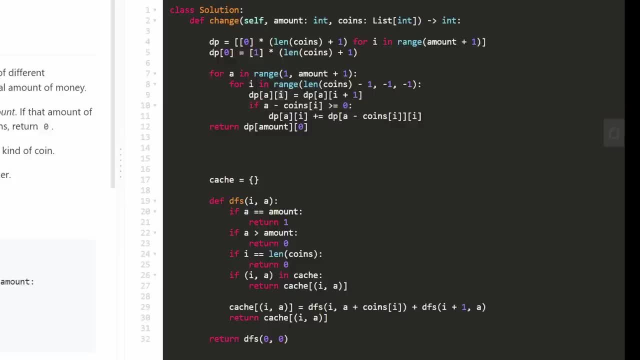 but so suppose we had this many coins available to us. that's what i says, and a we're trying to sum up to this particular amount. where, what? what is that going to? be well, one decision is: if we skip the coin at index i, which is just going to be dp of a uh with i plus, 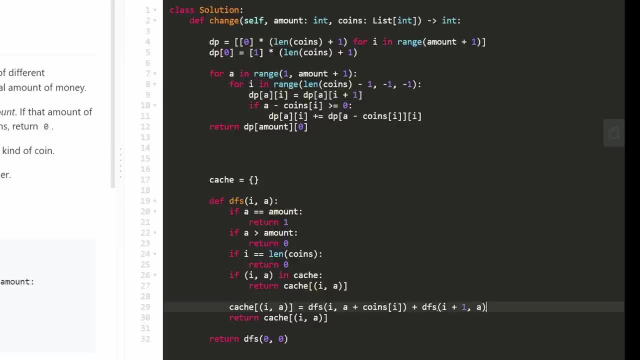 one. you can see that this line of code is the exact same. if you look below, this dfs is the exact same as this line of code, right, you can see the parameters are the exact same, right? all i'm doing is passing an a i plus one here. same thing here, right? a i plus one. now the other case is going to. 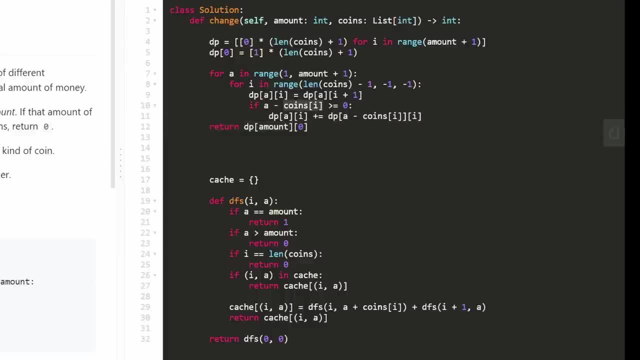 be uh with if we actually do use the coin at uh index. i right, so we're going to take a minus uh coins of i? why are we doing minus here instead of plus down here? well, you could do it. you can implement it how you want. i did it like this because uh a is the target amount if we use. 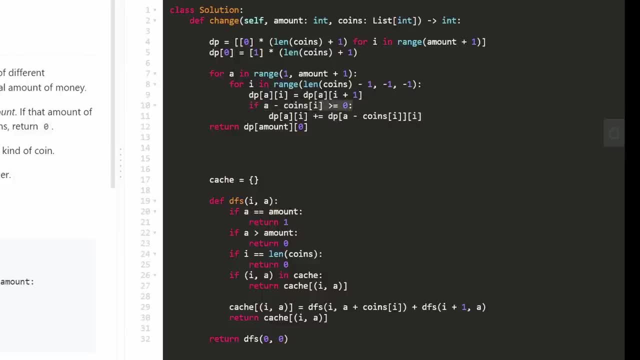 this coin, then we have a certain amount left over. now we're confirming that whatever that amount left over is greater than or equal to zero, because if it's negative, that means we went over right, that means we use too many coins. so if this is greater than or equal to zero, then this line of 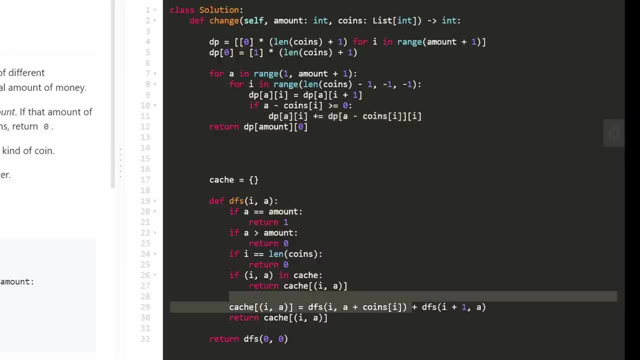 code is just, is completely analogous to this line of code, right? so if we use this line of code, this dfs down here, if you can see it, this dfs where we pass in i, uh, a plus coins of i, you can see that instead of passing a plus coins of i, i'm doing a minus coins of i. right, but this is uh, if. 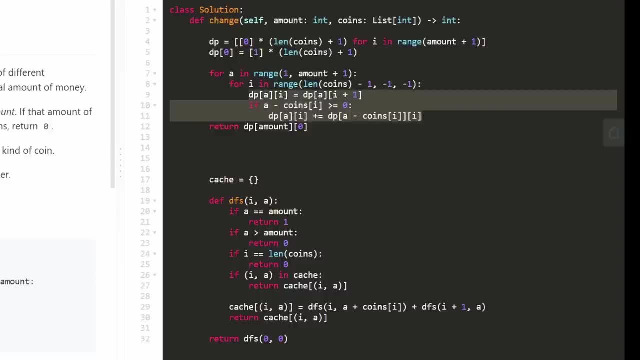 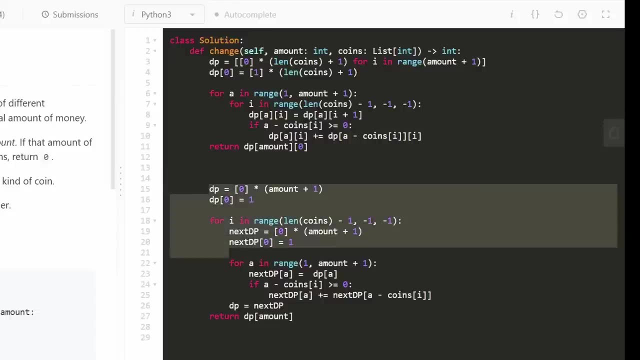 you get confused by this, i would recommend going back to that two-dimensional grid that i was showing you, because this is exactly the same as that now. last but not least, i have went ahead and copy and pasted my code for the solution where the memory complexity is actually just big o of n? the 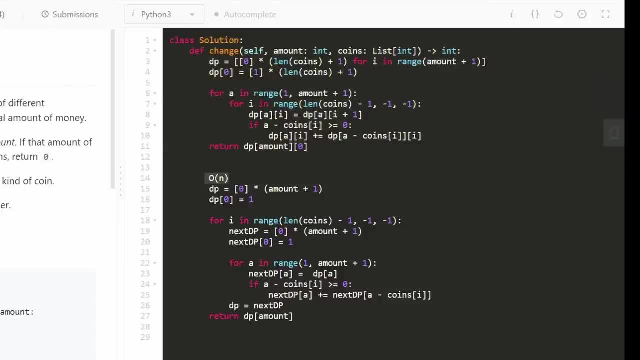 complexity is the same as the above solution, but the memory complexity is less. you can see that that's exactly what i'm doing here, right, we're not actually using the full, uh, memory. we're not using two dimensions of memory, we just have one dimension and you can see, just like in the 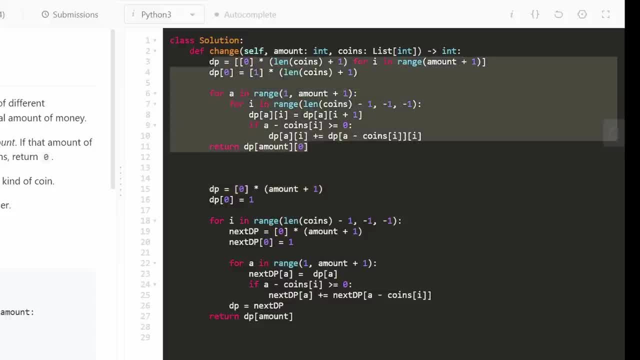 two-dimensional matrix that i showed. the main difference between the above solution and the below solution is just the order that we're computing the uh, the two-dimensional grid, right, you can see, in this case, the outer loop is we're iterating through the amount and the inner loop. 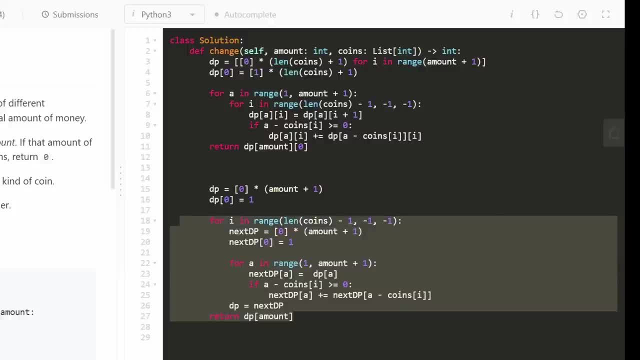 is where we're iterating through the coins. in the other case, the outer loop is iterating through the coins and the inner loop is iterating through the amount. but other than that, the entire solution is pretty similar, right like here. you can see, i'm pretty much just i have one row that i'm 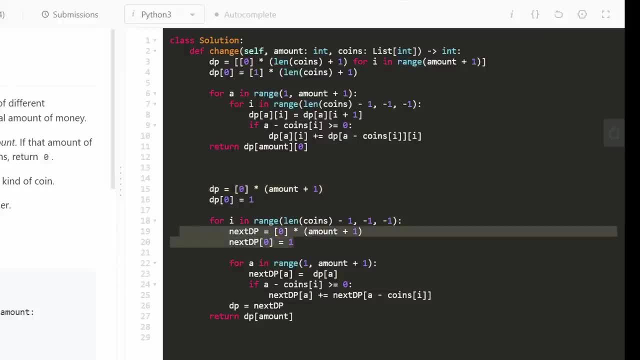 maintaining out here and then i'm i'm using next dp to be the next row that we're computing and then at the end i'm just reassigning dp to be next dp right at any given point. we're only going to in memory. we're not going to have an entire two-dimensional grid. so i know this was really. 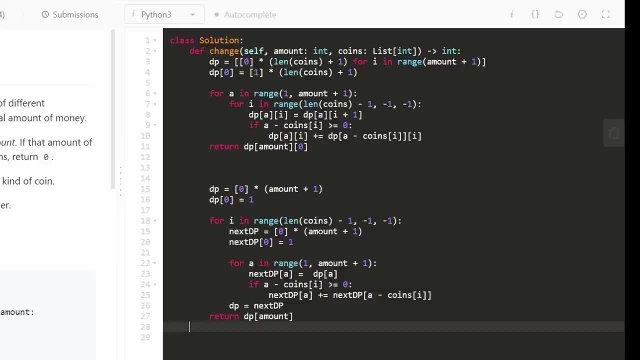 confusing and this is probably a long video. i wasn't able to spend as much time on the code as i would like, but i hope that the drawing explanation was able to help you out. this code will be in the description. if you want to take a look, i guess let me just run it and prove to you. 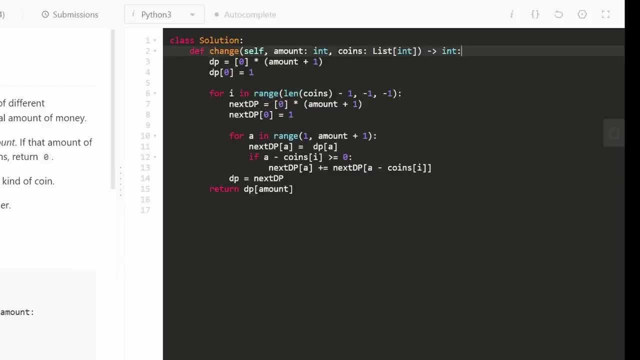 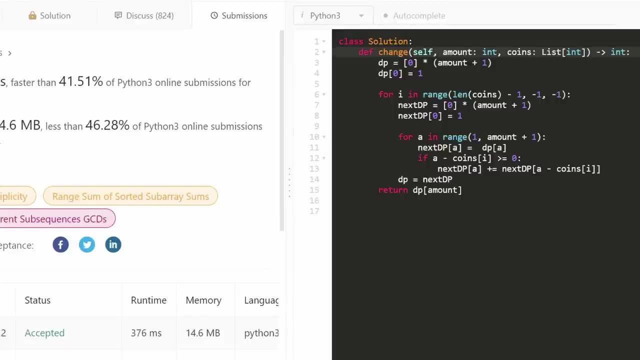 that it works, so i'll run the code that is below, which is the most optimal solution that i was able to come up with the time. complexity is n by m and the memory complexity is o of n. you can see on the left that it does work, so i'm going to run the code that is below, which is the most optimal solution. 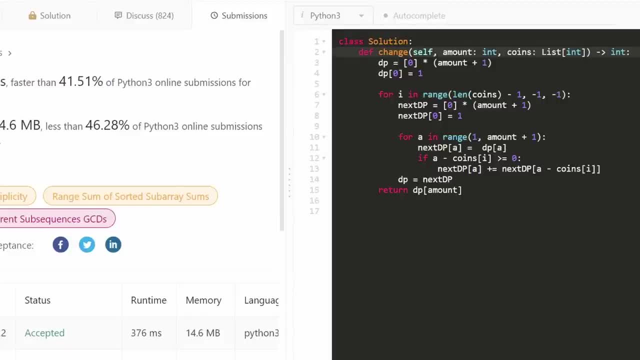 and it's pretty efficient, so i hope that this was helpful. if it was, please like and subscribe. it supports the channel a lot and i'll hopefully see you pretty soon. thanks for watching.